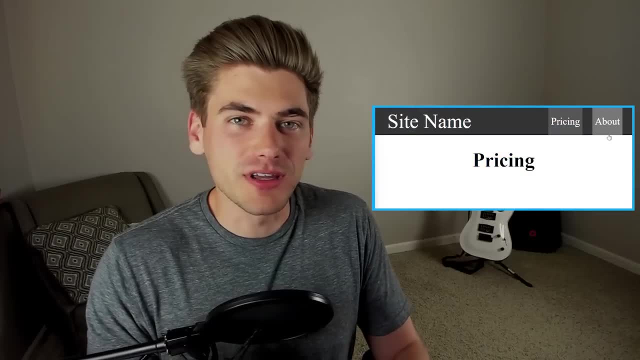 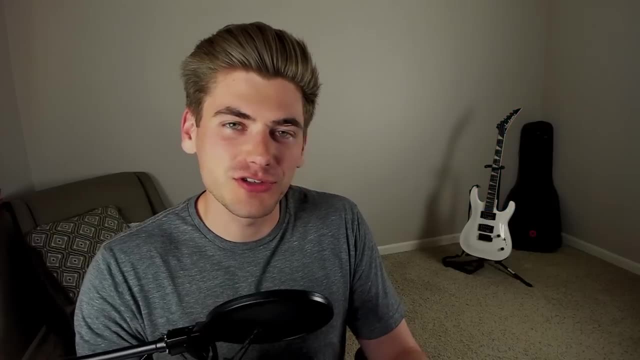 In today's video, we're going to create this fully functional navbar in React which has active link highlighting and properly refreshes only certain parts of the page. And, best of all, I'm going to show you how to do it using React Router and without using any router library at 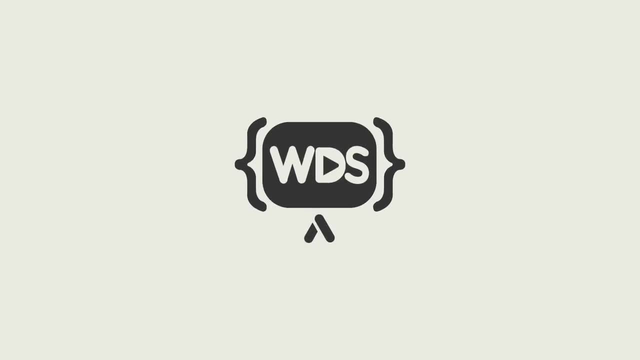 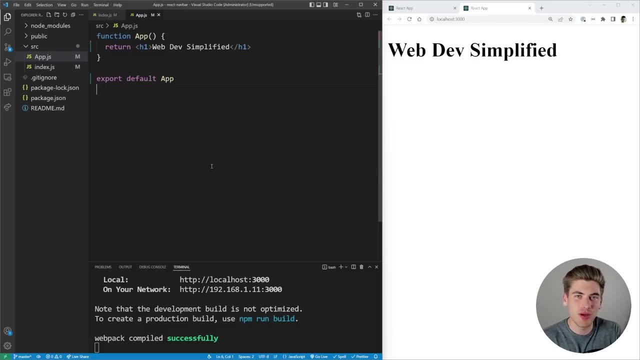 all so you can truly understand exactly how this works. Welcome back to Web Dev Simplified. My name is Kyle and my job is to simplify the web for you so you can start building your dream project sooner. In this video, we're going to create the navigation that you see here, where you have 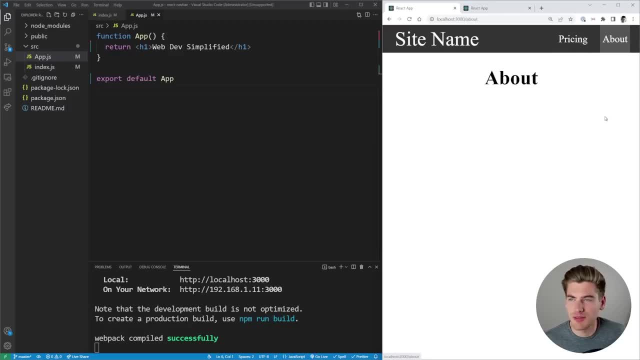 different links. We can click on them and you can see that the active link is highlighted. Same thing with the Zip Out page, And then we can go back to the homepage- Really simple navigation. I'm going to show you how to use React Router to create this, and also how to create it without. 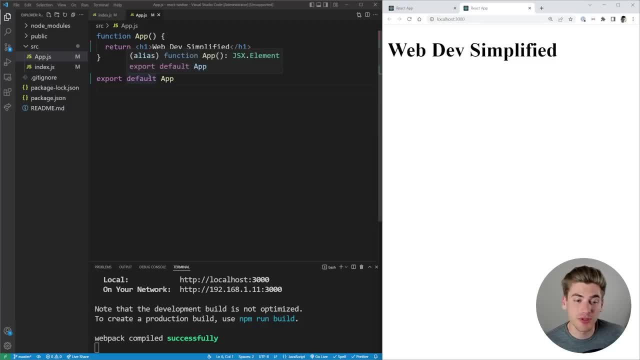 using any router at all. So to get started, I just have a boilerplate: create React application. I deleted out all the code we don't need and we're just left with a simple H1. Now to create this really simple navbar. we're just going to create a component for it. We're just going to call this: 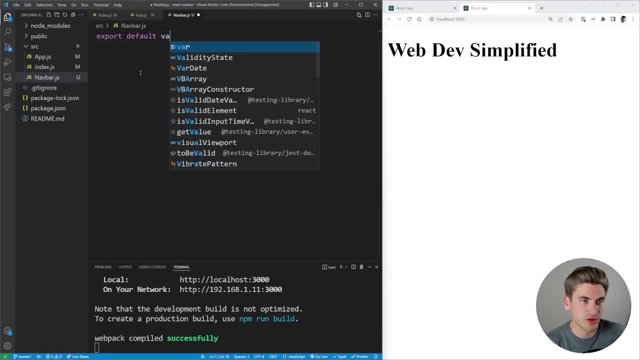 navbarjs, And in here we're just going to export H1. Default function, which we're going to call navbar, And inside of here is we're going to put all of our navigation code and it's going to be really pretty straightforward. It's just going to 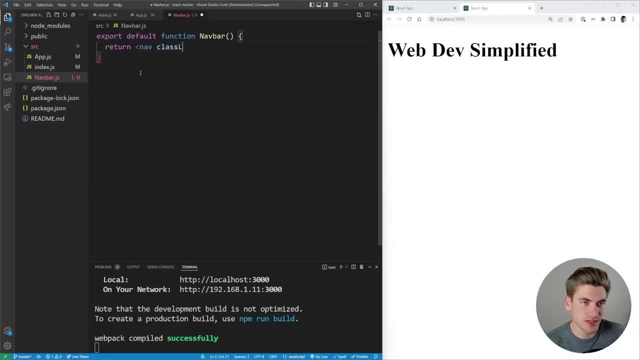 be some JSX. So we're going to want to have a nav element, which I'm just going to give a class here that we can use this later. So we'll give it a nav class And then inside of here I want to have a. 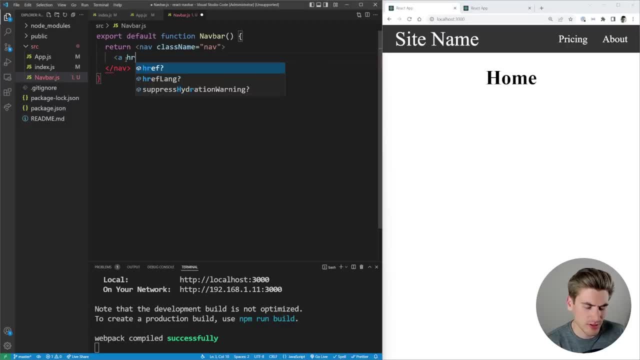 link for the left hand side. So this is going to be our site over here. That's going to be a link that leads to our homepage, just like this, And we're just going to call it site name. You can call this whatever you want. Also, I'm going to give this a class so we can style it specifically. 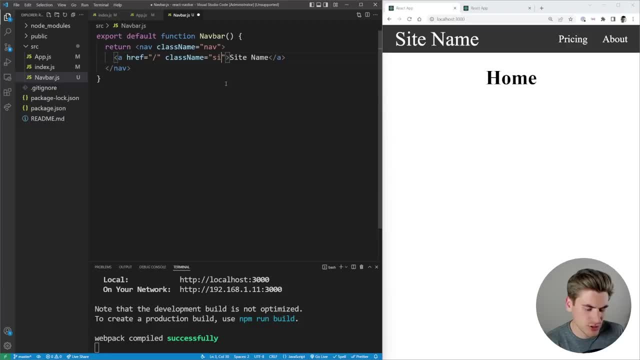 because I want this to be styled with- you know that like larger font. So we're just going to call it site title. Then, below this, we're going to have this list on the right, And generally, when I'm doing a navigation like this, I like to use an unordered list. So I'm going to use an unordered. 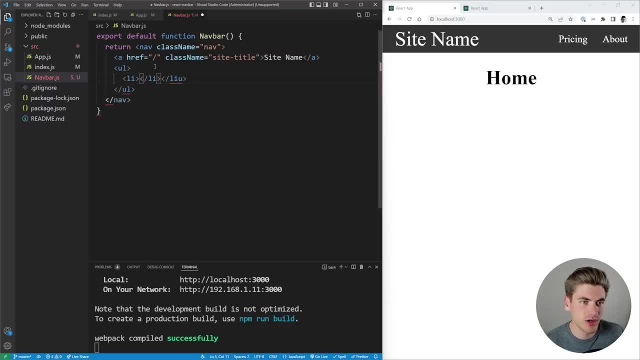 list And inside of here I'm going to have an LI element for each one of the pieces of my list. Inside those LIs I'm going to have an anchor tag and that anchor tag is going to have our href. So, for example, we're going to have our pricing page And that's just going to say pricing inside of 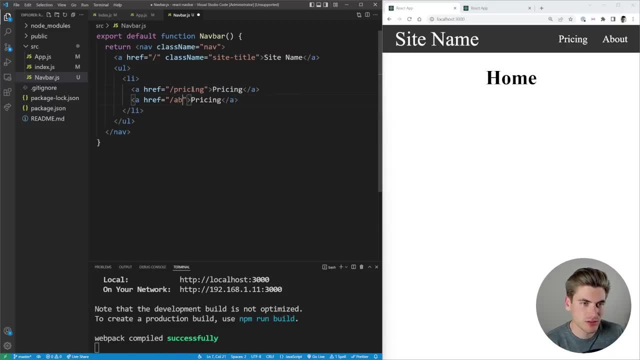 here, And then we're also going to have an anchor tag, And that anchor tag is going to have our about page, which is going to say about: just like that: Now if we go into our app real quick, we can just render out that navbar component, So we can just come in here and say: navbar. 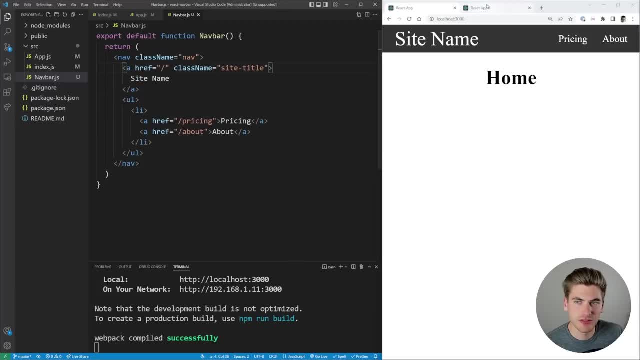 make sure that that gets imported at the top of our page And if we save both these files and we come over here, you can see we have our navbar, But obviously it's not styled how we want it to be And also it looks like I forgot to put each one of these in their own individual. 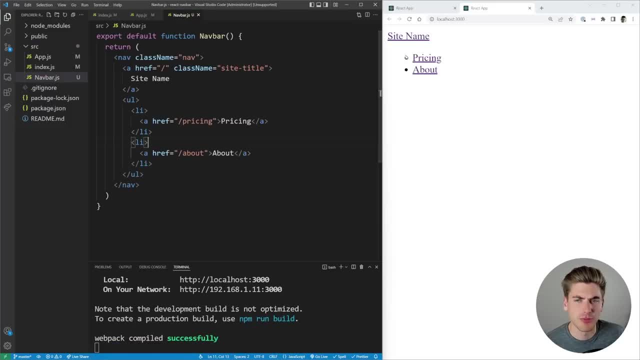 LI. So let me make sure I do that real quick. There we go Now. they're both on their own LI, So now what we need to do is actually make this styled correctly. So I'm just going to use a simple stylus sheet for that. I'm just going to 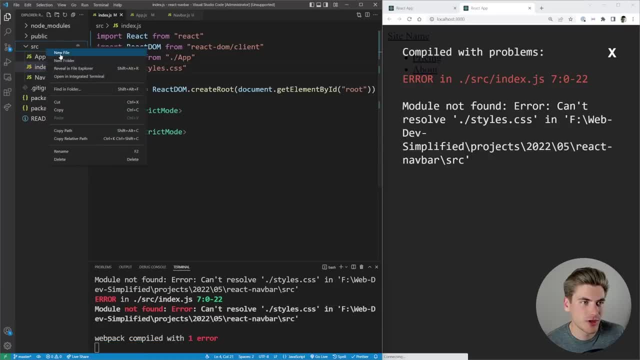 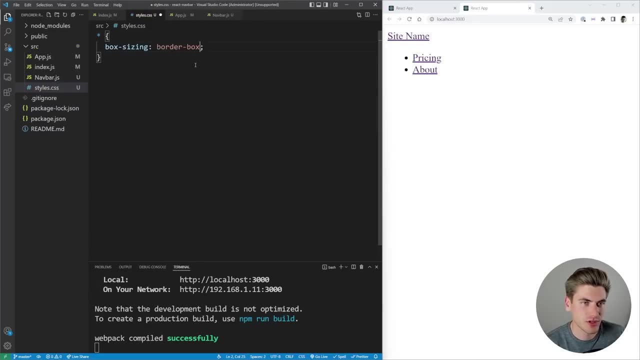 import stylescss And I'm going to create that stylescss file And inside of here, the very first thing I like to do is just to set up my box sizing. So we're going to use border box And on my body I'm going to say that there's going to be no margin. Now, with that done, 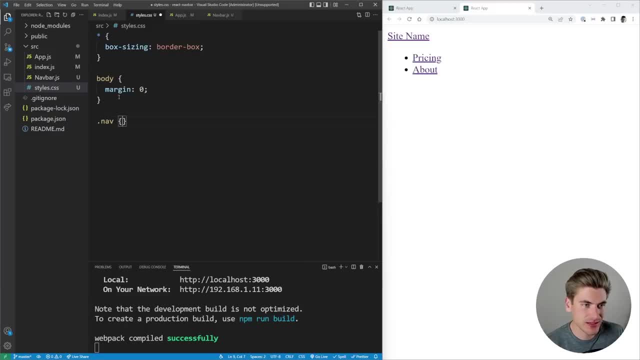 we can work on styling out our nav. It's going to be pretty straightforward. Let's select that nav element. I'm going to give it a background color here, which is 333 and a color of white, So the text is going to be white. 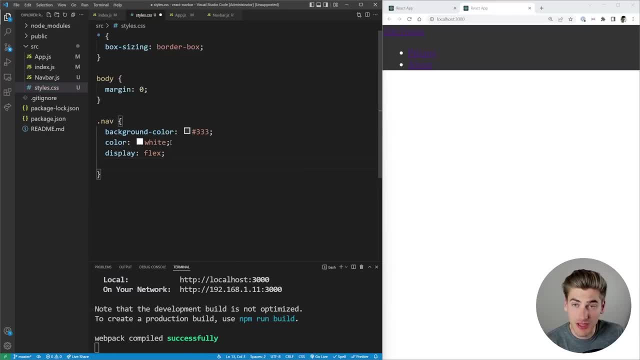 Next thing that I want to do is I want to make sure I use display flex here, And that's going to allow me to space everything out how I want it, So, for example, I can justify my content with space between- And that's going to push these different elements to the left and the right. 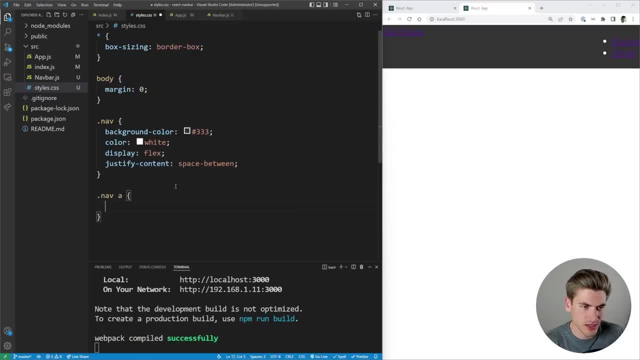 side of the page And in order to make the link show up, let's just select those anchor tags. make sure that the color here is set to inherit. There we go, So we can see those white links. So you can now see they're pushed to the sides And if I use align item center, that's going to center. 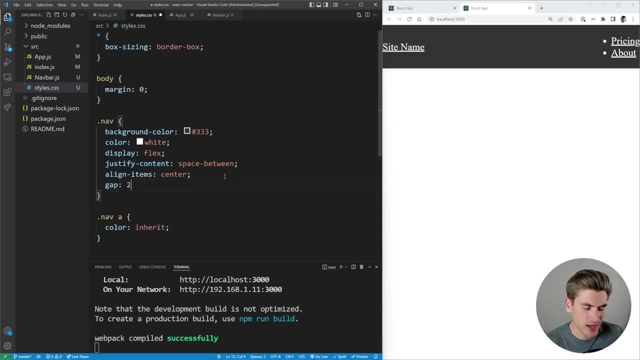 them vertically, which looks really good, And then what I can do is I can specify a gap of two REM and then some padding on the left and right of one REM, So the gap puts space in between my elements. So if they get too close together there'll be space between them, And then 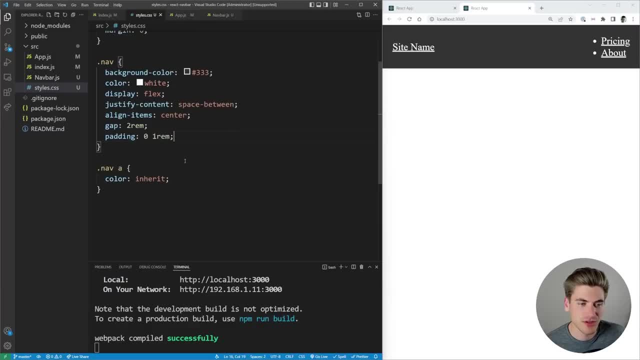 the padding is giving me space on the edges, so they aren't quite touching the edge of the screen, And the next thing I want to do is I want to make it so that these links and such look a little bit better. So in order to do that, what I'm going to do is I'm going to come down, I'm going to take 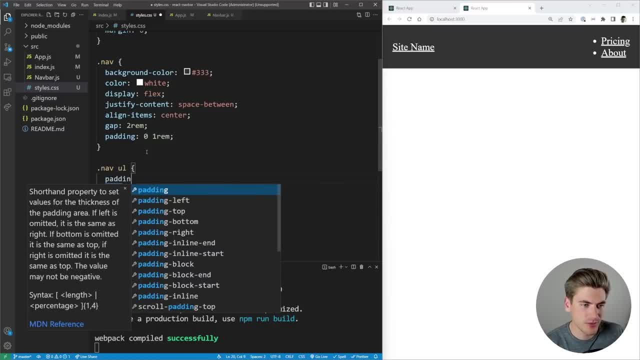 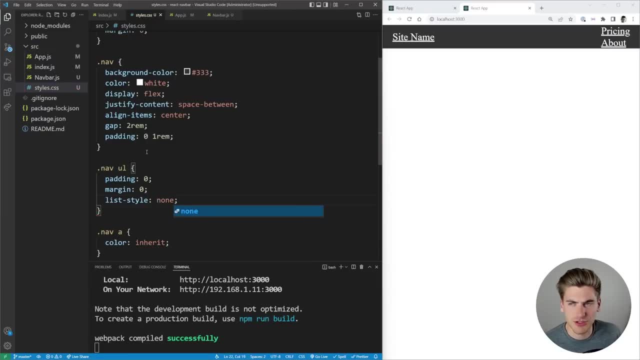 my nav, I'm going to select the UL itself. I'm going to get rid of all the padding and the margin that are on here by default, And then I'm going to say that the list style is going to be none. That's just going to get rid of all the extra spacing and get rid of that circle. on the 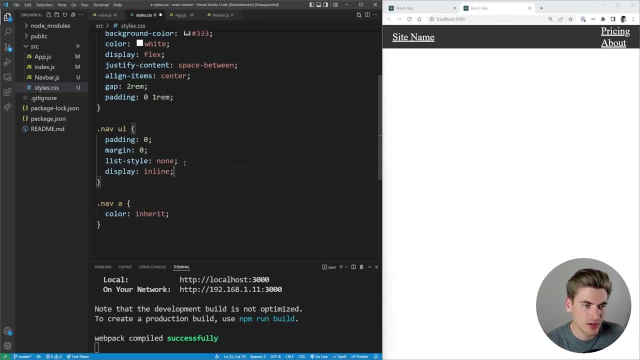 left hand side of my different list elements. That looks really good. Also, I'm going to specify this as a display flex with a gap of one REM, And that's just going to put some space in between these different elements. Now, if we move down, what we can do is we can actually start styling. 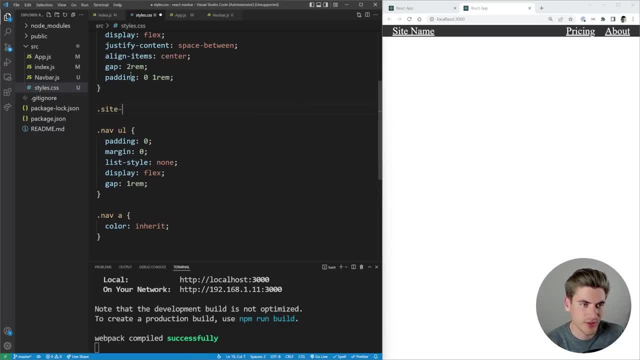 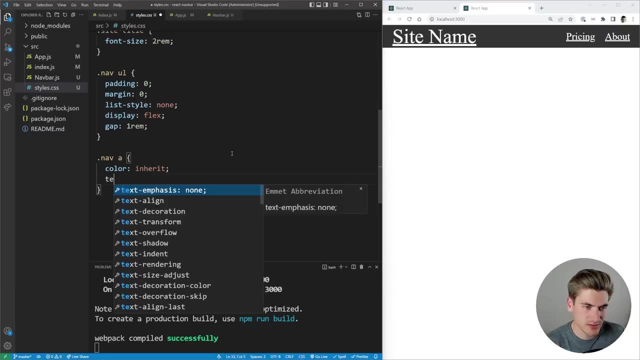 out our nav itself with this anchor tag. But also I want to style out that site title by just increasing the font size to REM, so it's a little bit bigger. Now, on our actual anchor tags, text decoration should be none, because we don't want those underlined. And then I'm going to go ahead. 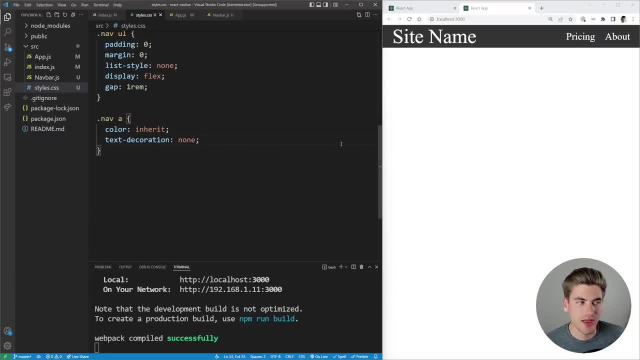 and do the same things on the left hand side of the anchor tag. So AXELA and I, if you look here, we have two text designs that looks a lot better already. And now what I want to do is I want to work on that active class, making that work. So what we're going to do is we're going to take our 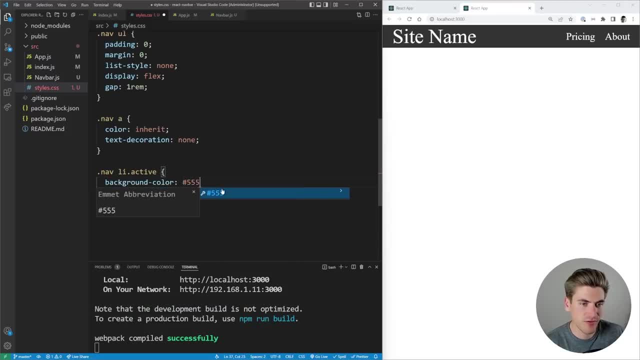 nav here, And what I want to do is: I want to get the Li that has the active class on it. I'm going to specify a background color of whoops 555.. And then on hover I want to have a different. 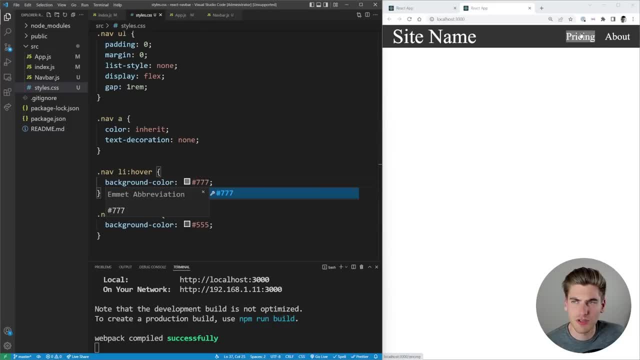 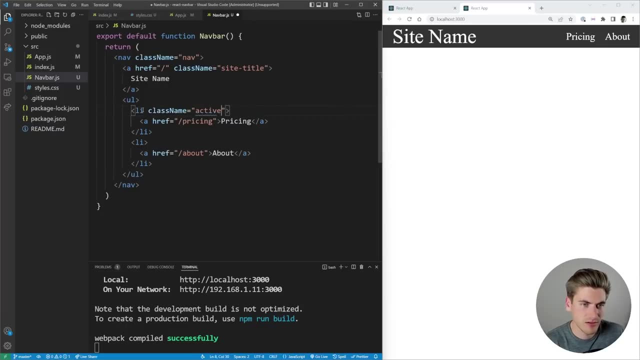 background color. So if we come over here we hover this, I want to have a background color of 777.. So now, if I save when I hover over these, you can see they get that background color And if I li, you can see that it now has a different background color. but you'll. 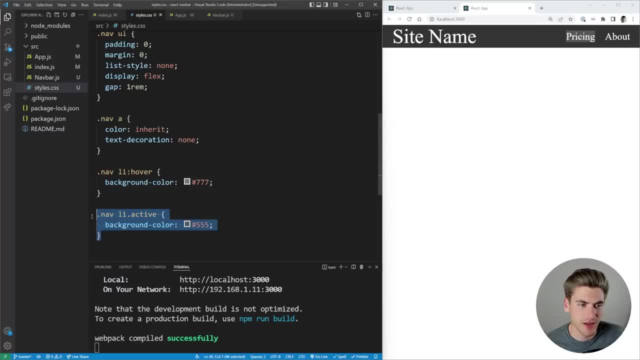 notice that the actual height is not quite right. and also I should make my active class go above my hover, so that way when I hover the active one it'll change the background color. there we go now. I just need to make sure that this is essentially full hikes. right now my link right here is not full height, so we 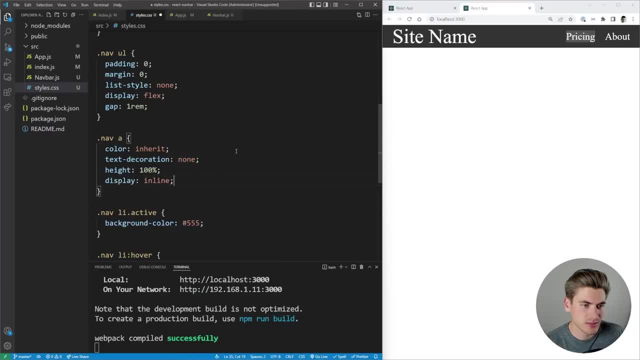 can change this to a height of 100%. whoops, a display here of flex and we just align our items in the center. that'll make sure our text stays in the center, and then we can just give some padding to it, which the 0.25 REM now as 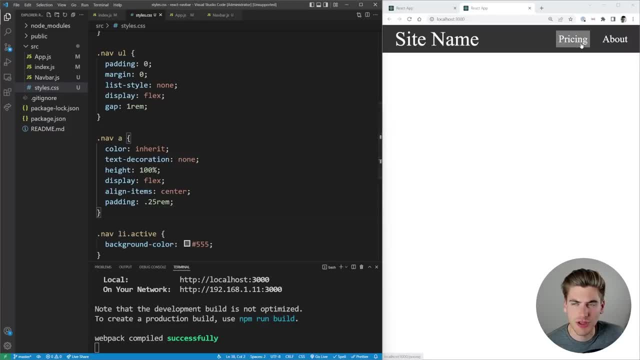 you can see that worked a little bit. the only thing we have left to change is to make it so that our actual ul element spans the full height and we can just do align items of stretch, and that should actually fix that for us. and there we go. 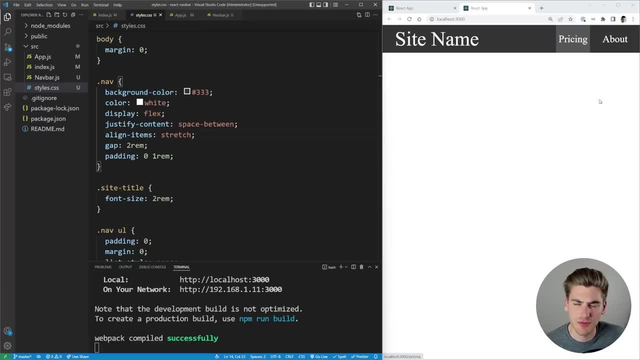 that works perfectly. so now, when we hover these, we get this nice highlight effect and whichever ones active has that background color being applied to it, so it's like the really basic styles we need. you could obviously make this look much better, but the real core here is that we have this active class that 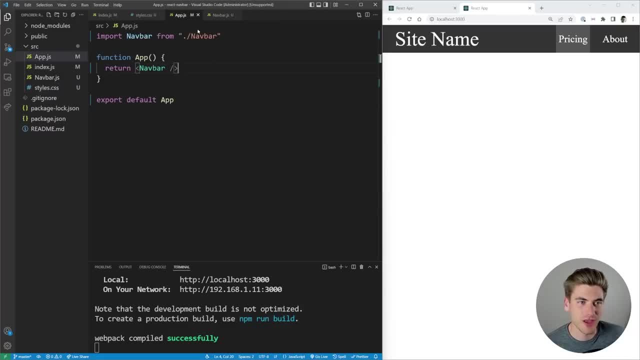 does something, so that way we can use that inside of our JavaScript and our react code. so, now that we have our navbar, what I want to do is I want to create some pages, and these pages are going to be the text of home pricing and about so. 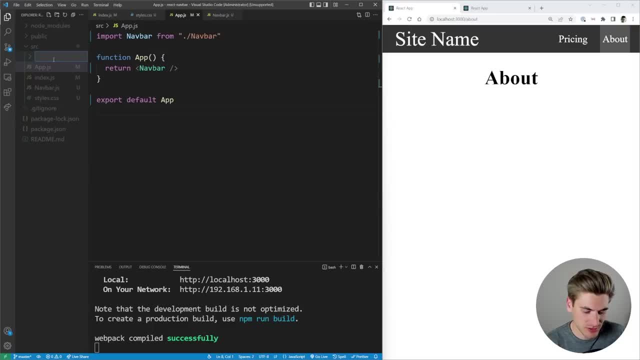 there's gonna be separate components that contain all of our code for that page. so let's create a folder called pages and inside here I'm going to create a new file. we're trying to call this one homejs, and inside of here export a default function called home, and all this is going to redo is return an h1. 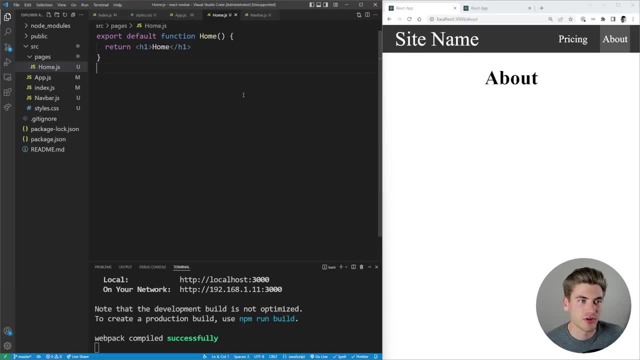 with the text home inside of it- really super straightforward. I'm going to do that for all of our different pages. so we have here our about page and we also have our pricing page, and inside of our pricing page I just want it to say pricing and instead of home or instead of about, I want it to say about. 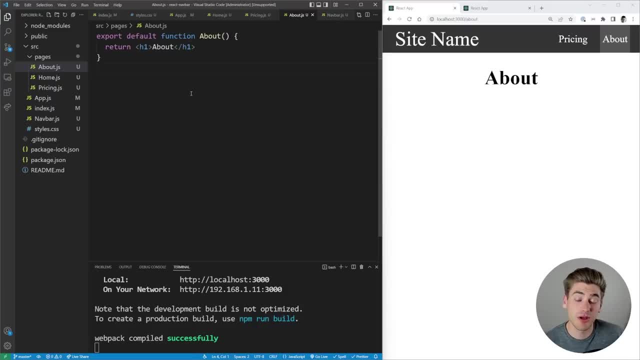 so now we have three different components, one for each of our different pages. I want to render out those components dynamically, depending on what page we are on. so right now, when we click on these links, you can see it refreshes our page and then our URL changes to slash pricing. so inside of 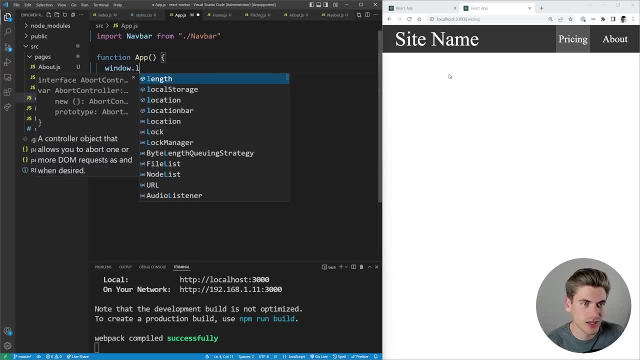 our app. here we can actually get the URL on our page by saying window dot location. so if I just console log this out, you should see here. if I inspect my page and bring this over, we look at our console. you can see our location here has a bunch of information but most 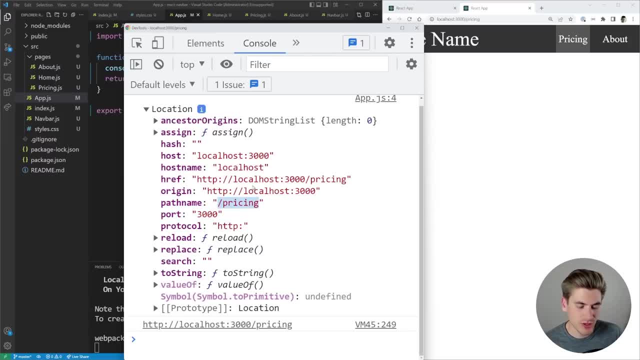 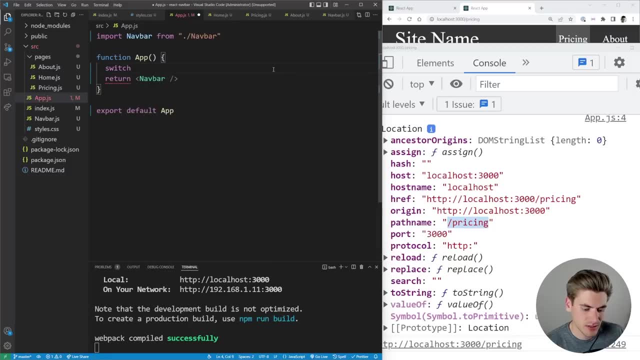 importantly, we have our path name, which is set to slash pricing, so we can really easily just take this path name and do a simple switch statement over it. so we can say here that we want to do a switch statement and this switch statement is on our window- dot location, whoops location, dot path name. and here, if we 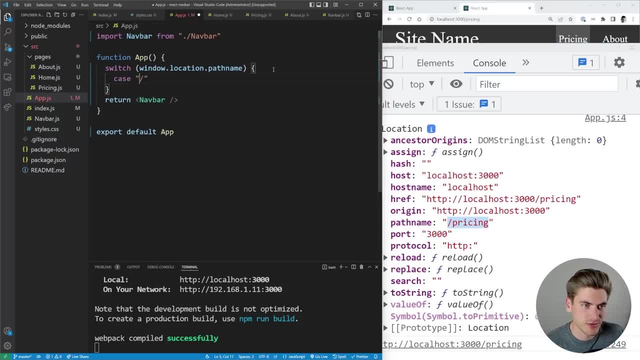 have the case where it's just going to be the home page. we're going to do something specific, so I'm going to put that in there with a break. then what I'm going to do is I'm going to say: hey, you know what, if we're on the pricing page which is slash, 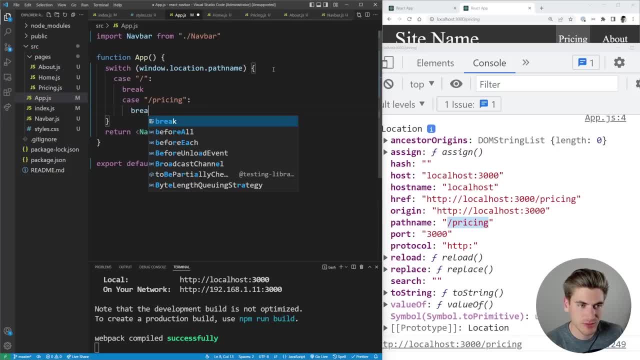 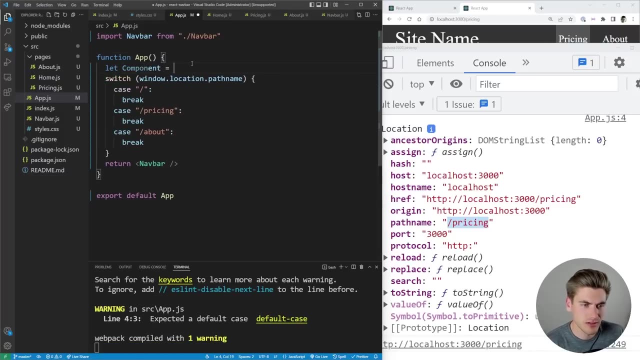 pricing, then we're going to do something else specific and break, and then finally we have our slash about page and we're going to have a break here as well. so now for our different pages. we just want to create a variable- let's just call it like component, and it's going to not be equal to anything by default, and we want: 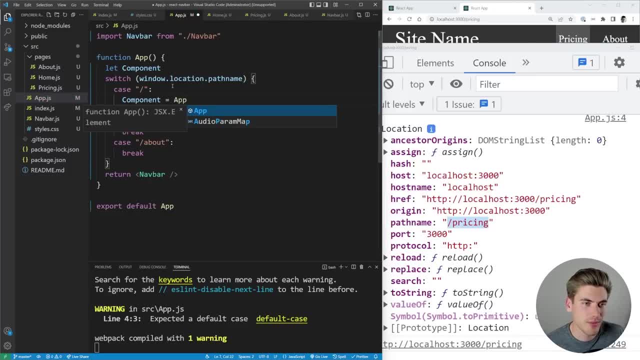 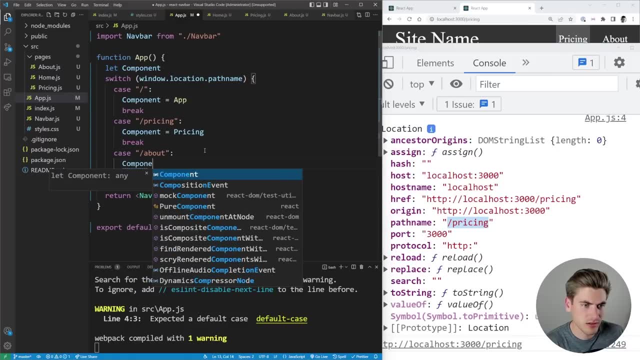 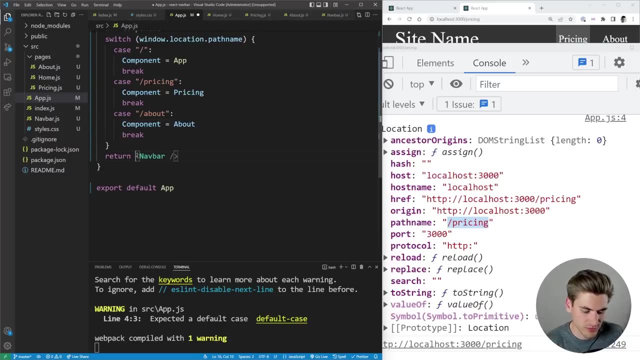 to do in here is we're going to say: you know what component here is going to be equal to our app, and down here, our component is going to be equal to pricing, and down here, our component is going to be equal to that about page, and then we can just render that out. so we'll just come to here. 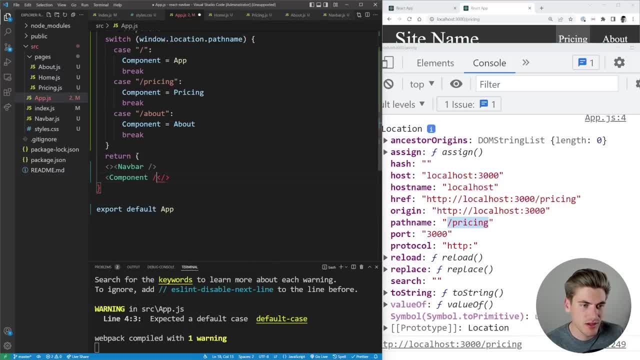 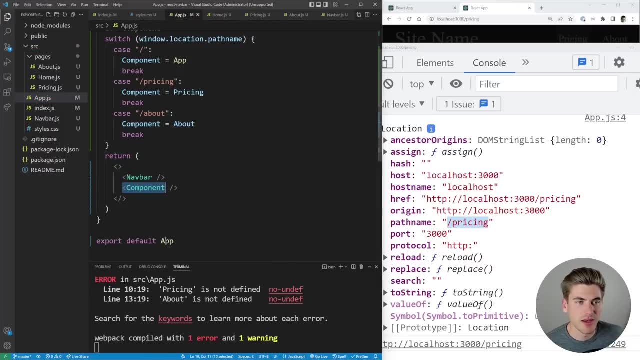 and we're just going to come down and render our custom component. now. one thing that is important to make sure that you understand is, if you are using these custom component, that you need to render out by name and then click on the by name. you need to make sure you use a capital letter, otherwise it's going to try to render out. 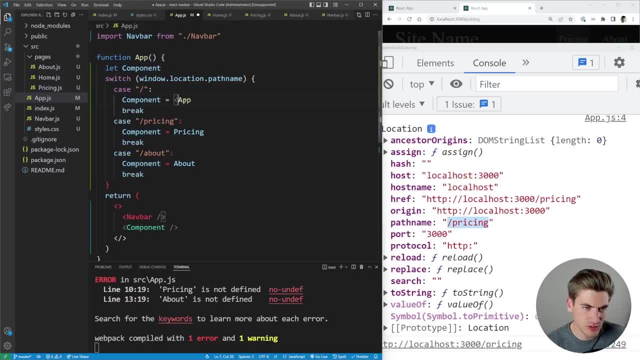 a normal html component, which is obviously a problem. otherwise, what you could do is you could say that you know, you have your app here, you have your pricing here and you have your about like this, and we could just call this anything. you know, it could be a lowercase component in that case. 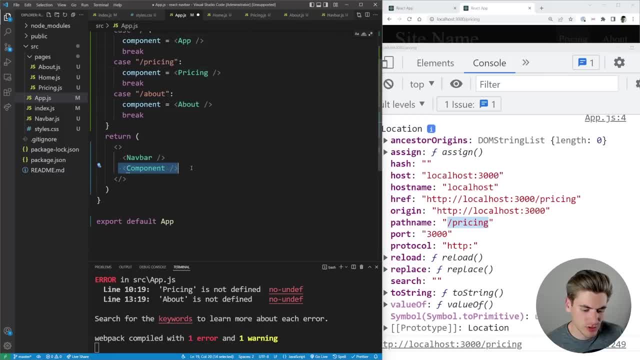 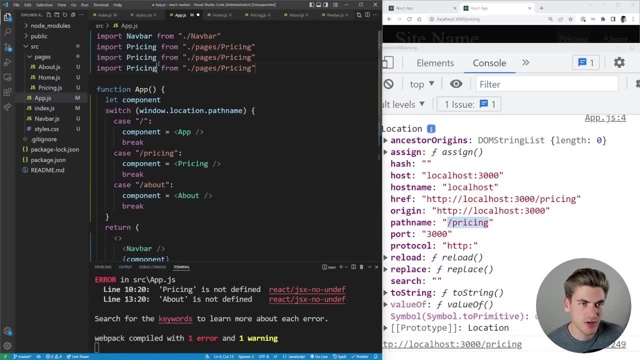 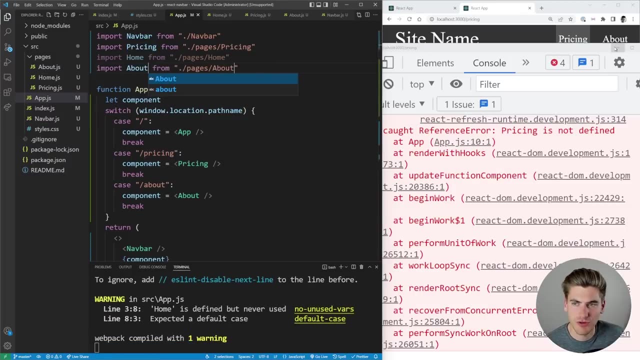 let's replace all those and then down here we would just render that out like this: so either way is going to work. we'll just leave it like this for now. now all we need to do is import all those pages that we just created. so we have pricing home and about. so now, if we come back over into 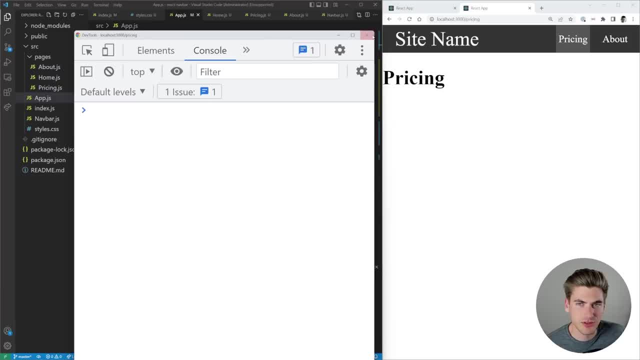 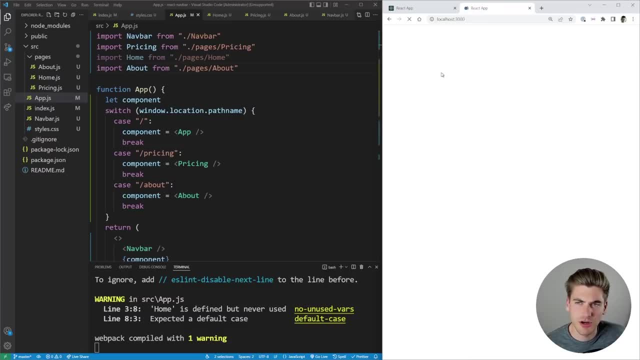 our application. we have some errors. it looks like. we'll just clear those out. refresh to make sure. now those errors exist, as you can see they don't. and now we have our pricing being shown. if we go to about, you can see it says about. and if we go to our home page, if we just give it a second to, 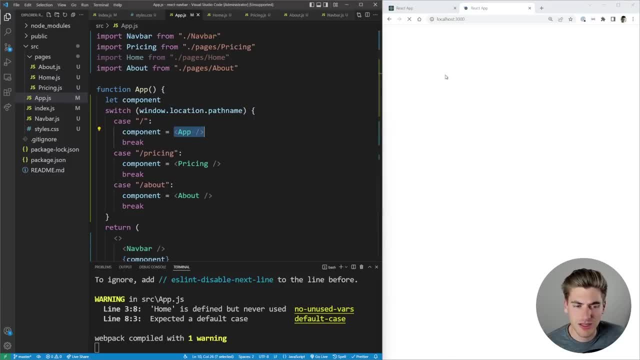 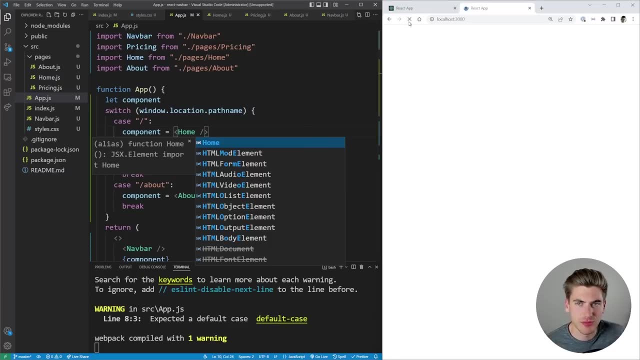 load here. it shows so this app right here, but it looks like we have maybe an infinite loop or something going on. it actually looks like the problem is i just put app here instead of home. that is giving us an infinite loop. so now, if we just bring this onto a new tab there, you can now you. 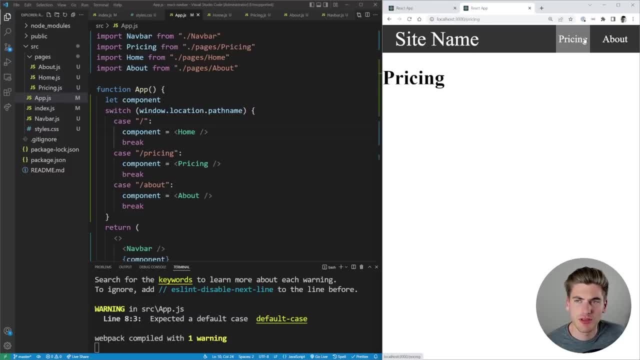 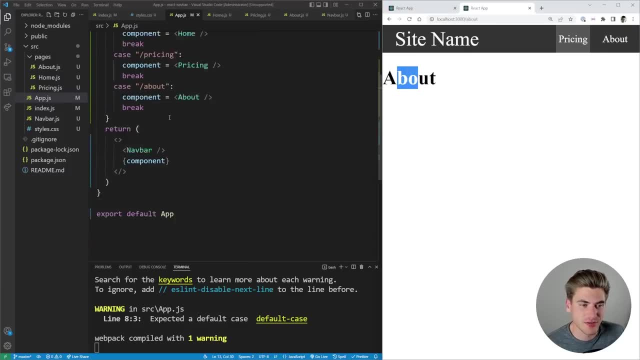 can see- i close- that we have our different pages showing up properly. now we just need to make it so the active page is actually going to be showing up as the active one also. before we do that, i kind of want to put this text inside of its own little container, so we can just create a div here with a. 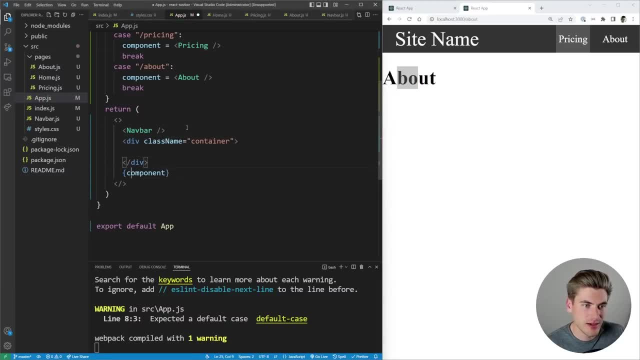 class name of container and then inside of that div we can render out this component and then we can go back to our css here and we can just scroll up to the top. we can say: dot- container. what i want to do is i want to give it some margin on the side, top and the bottom, and i 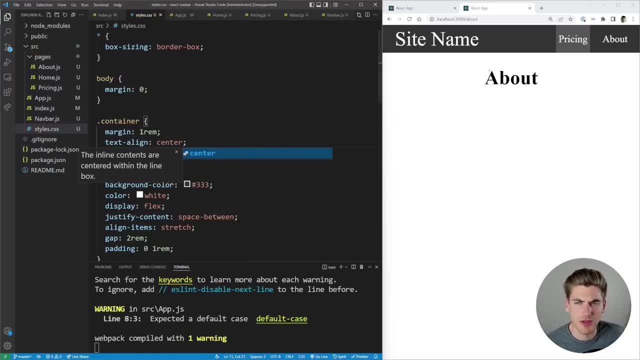 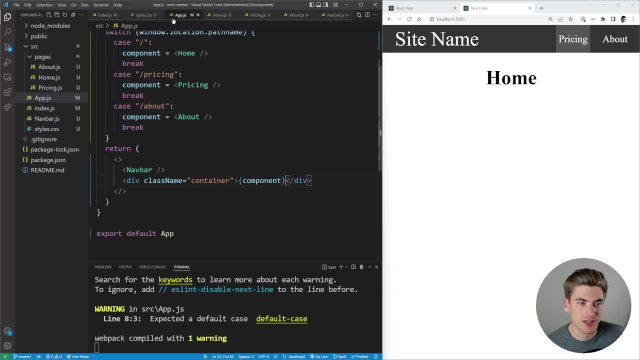 also want to text align it in the center. there we go, so now we have our text dead center. it just looks a little bit better. so now let's focus again on that active styling. the first thing that we need to do is we actually need to get that active page so we can just use this window dot location. 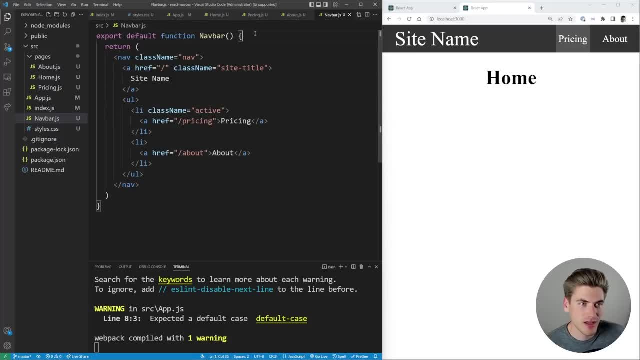 dot path name inside of our nav bar. we'll go into our nav bar and we have essentially our path, which is equal to this, and what we want to do is we want to see if our path is equal to this href right here. so we're going to go into our path and we're going to go into our path and we're going to. 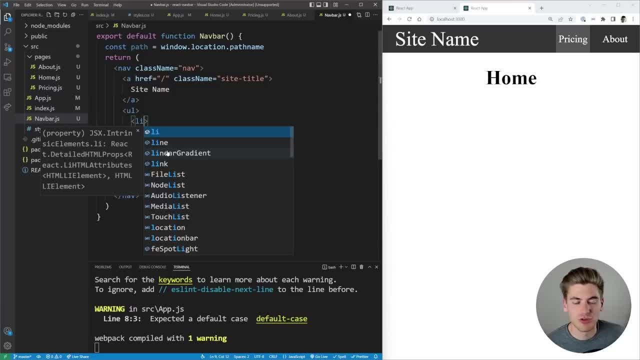 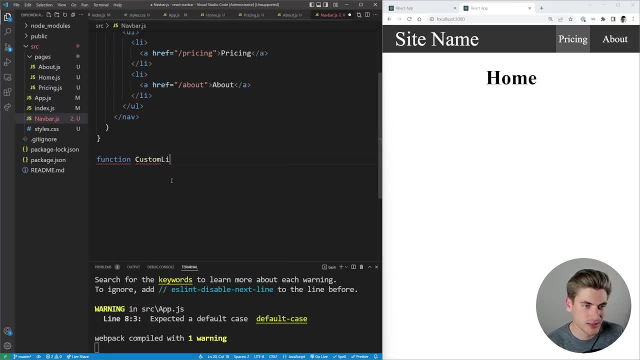 right here and that's how we're going to add that active class or not. so a really easy way to do this is going to be creating a custom component that wraps our link. so we're going to do that. we're just going to create a custom component. we'll call it custom link inside of this custom link. 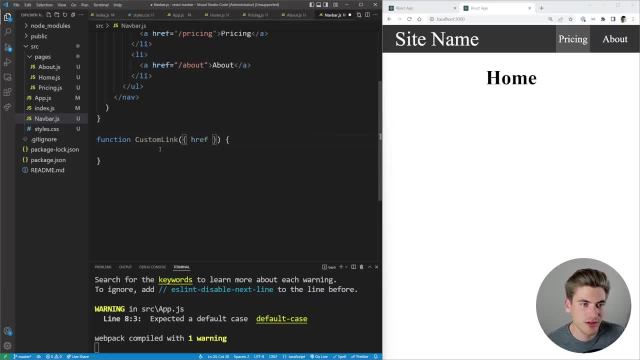 we're going to pass it in essentially an href, so we can just say href here and that's all we're really going to care. but we might also pass some custom props, so we're going to make sure we take those into account. so like, if we pass a class name along to here, we're going to make sure that. 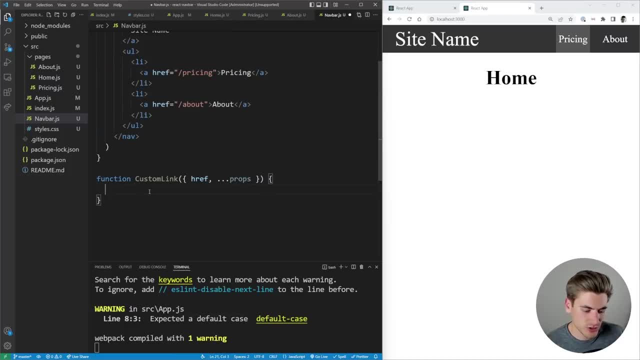 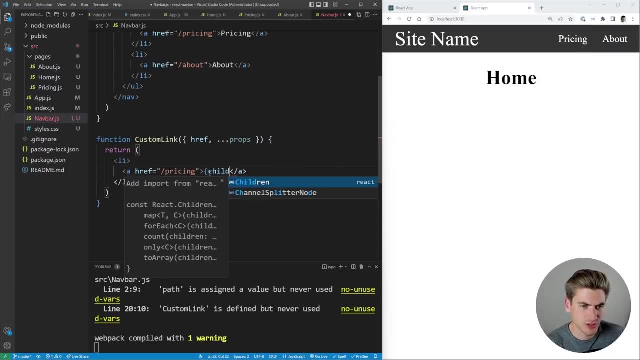 gets taken into account. so inside of this custom link we're just going to turn essentially our li with the link inside of it and what we want to do is we want this section right here to be our children, so we can come in here with our children and then we have our href. 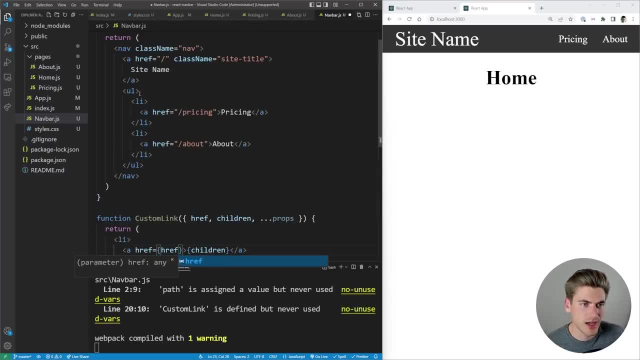 right here, which is just going to be equal to our href. so now i can essentially replace this with our custom link, and that custom link just has the text pricing inside of it- oops, if i can spell properly, and it's going to have this href being passed in as well, just like that, and i can do the. 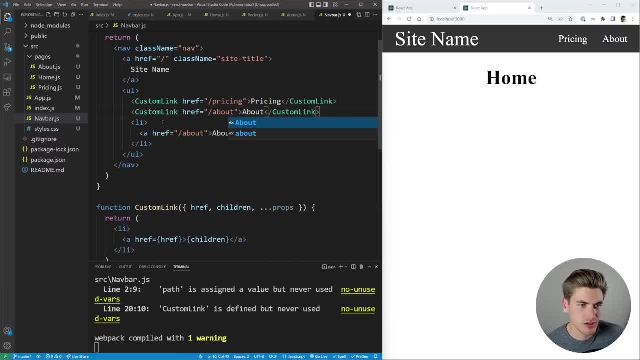 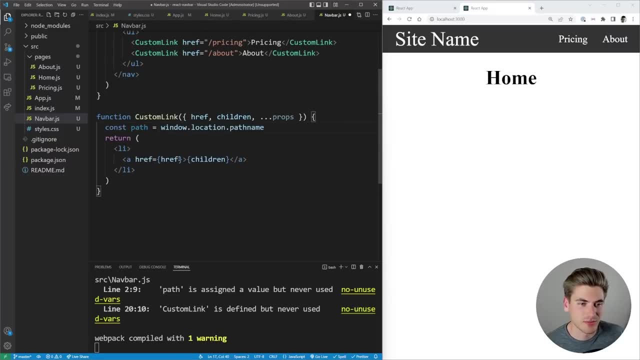 exact same thing for our href. so we're going to do that, and then we're going to have our href in our about page. so now all i've done is essentially simplified my code, and the reason i'm doing this is so i can take this path variable. i can use that inside of our custom link also. i. 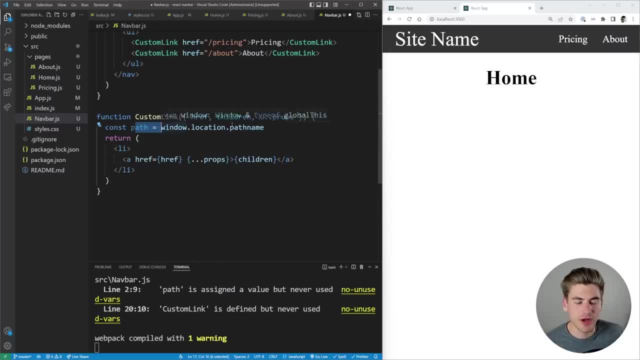 want to make sure i pass along any other props that we have. with this path variable i can determine is this the active path, because if our path is equal to our href and then we know that this is active. so what we can do is we can just take that code and we can say our li has a class. 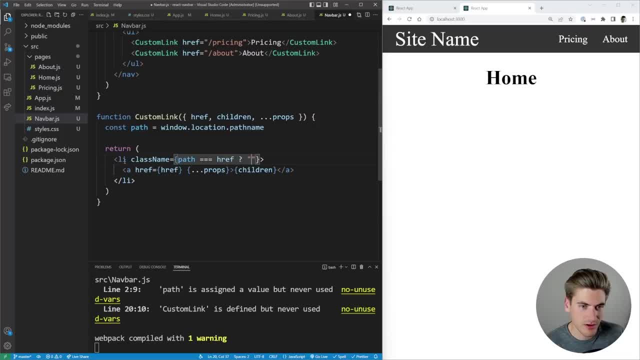 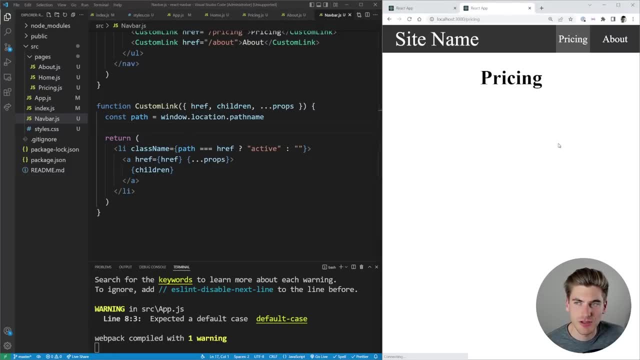 name, which is going to be equal to here. if these are equal, then our class is going to be equal to. otherwise, our class is equal to nothing. and with that one simple change. now, if we go to our pricing page, you can see that's marked as active. we go to our about page, you can see that's marked as active. 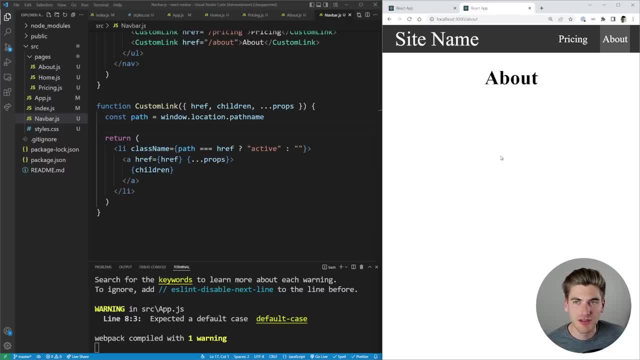 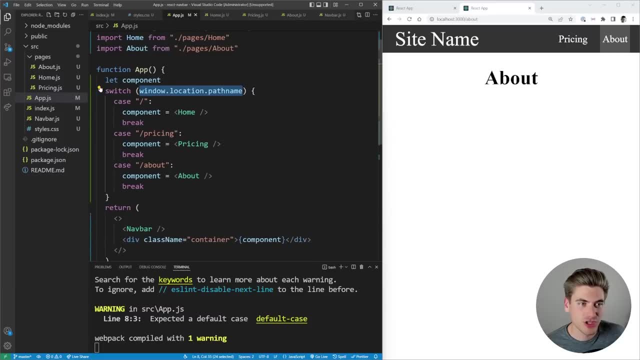 so no matter what page we go to, it's always going to be marked as active. now, obviously, this is not the most scalable solution, and the main reason for that is, if we go back into our app, here is we get this giant switch statement, which is not the most clean thing in the entire world, and every time we 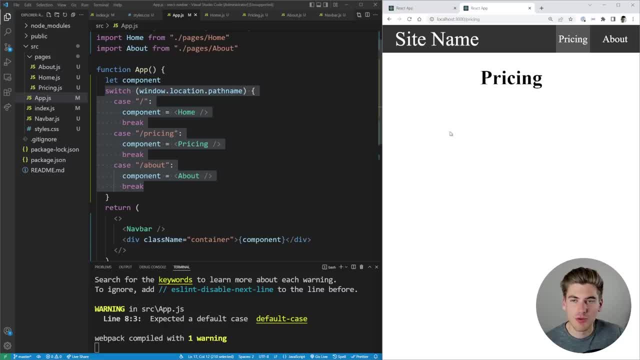 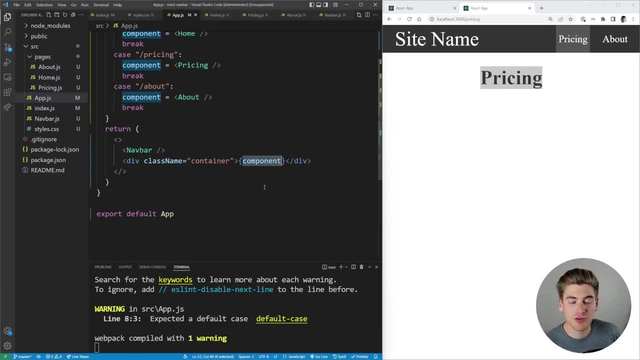 change a page, it actually refreshes our entire application, when in reality the only thing that changes is the component section. so we want to fix all that, and the easiest way to fix all that is by using a routing library such as react router. so in order to get started with react router, we're 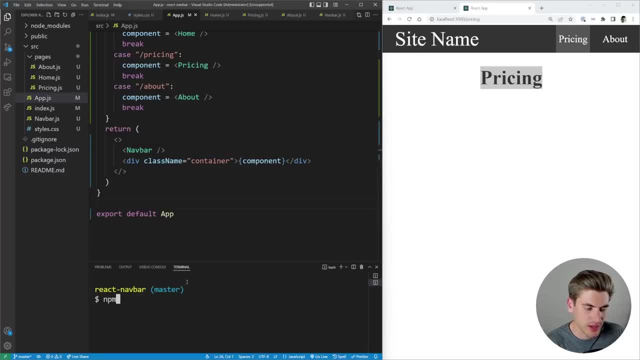 just going to come down into our terminal and we're going to install the react router library, and the react router library that we want is going to be specifically for the dom, so we're going to download react router dom, hit enter and that's going to download all the libraries that we need. 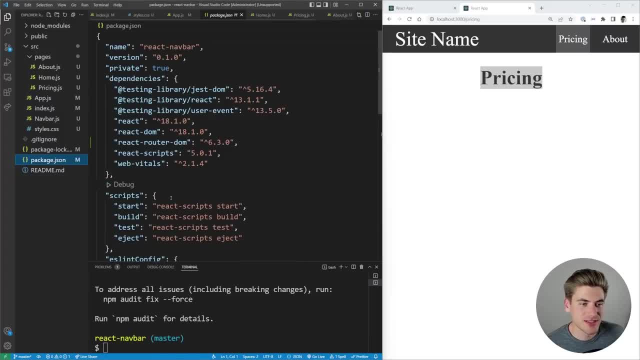 for react router. if we come into our package json, we give this a second, you're going to see right here we have our react router dom being installed, so we can actually use that now to use react router. there's a few things that you need to set up. first of all, you need 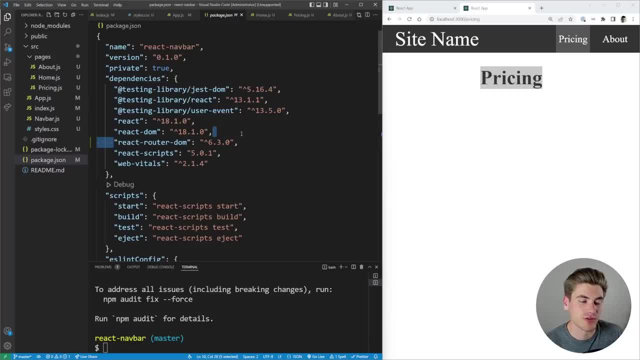 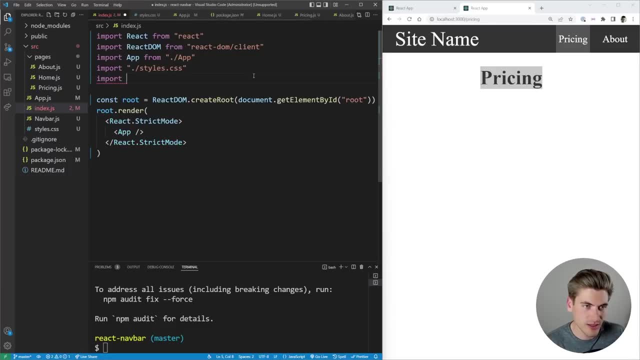 to set up what type of router you're using, and then you need to define all your different routes. what we want to do is we want to go into our index page, and here is where we set up our actual router that we're going to be using. so we're going to do a quick import here. that's coming from that react. 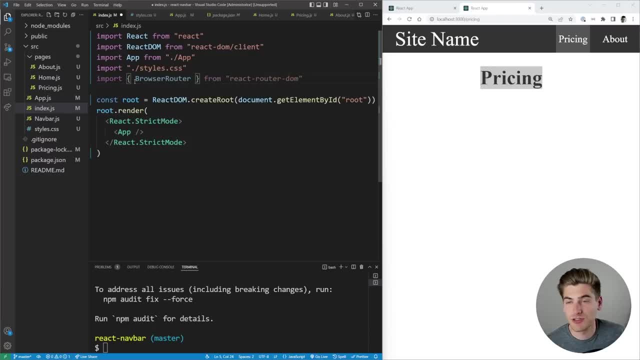 router, dom, and what we want to import is a browser router, and that's just because we're in the browser. react router allows you to do routing for things like mobile applications and so on, but for us, we're creating a web application in a browser, so we're going to be using the browser router. 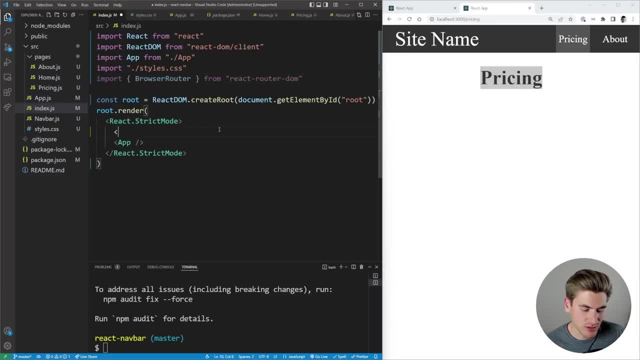 what you want to do with this browser router is just wrap your entire application. so we're going to come in here with that browser router and again we're wrapping the entire app component, because our entire component is going to be using this one single router to manage. 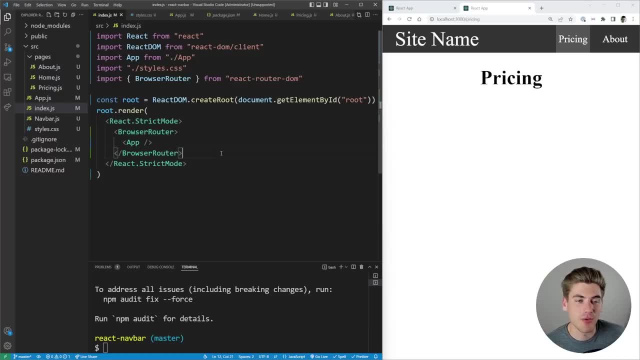 all of the routing. now the next thing we need to do is define that router and all the different routes inside of it. to do that, we're going to come in here and essentially replace this switch statement with react router code. so again, i'm going to come up here with an import statement. 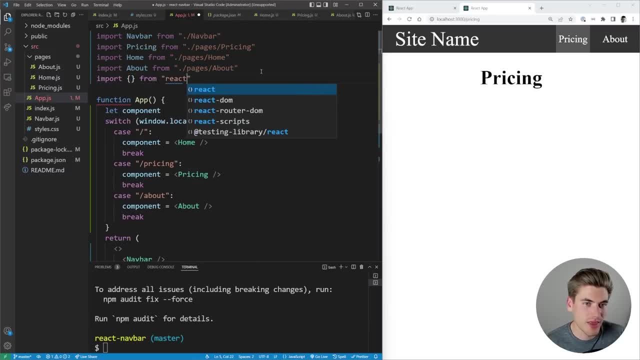 at the top and this is again going to be importing from that react router dom, and i want to import a route and i also want to import the routes component. these two components allow us to define all of our routes and group them together, so for now we can completely get rid of all of this. 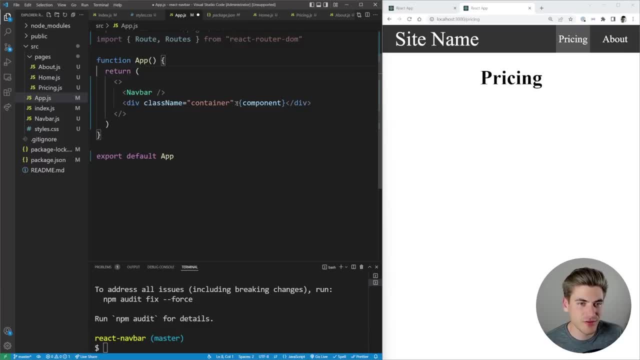 code right here, because we don't need any of this switch statement code, and instead inside of our container where we're rendering out our component. this is where we're going to use these two components of routes and route, so our routes component is going to wrap everything, so we're 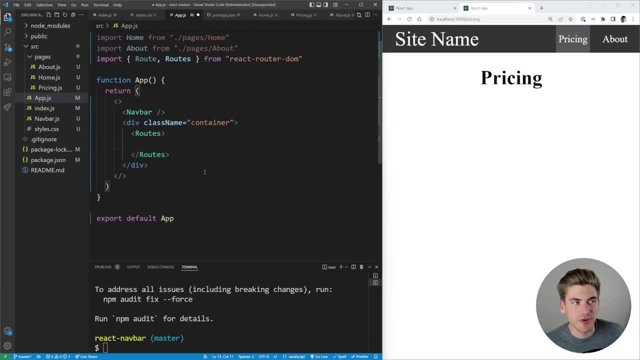 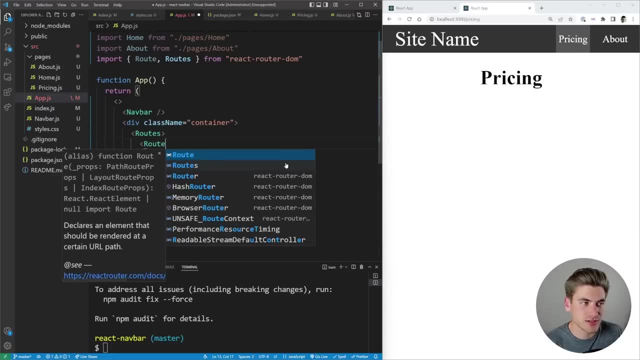 going to say routes and it's going to wrap all of our individual routes, and this routes component essentially just says: hey, here's a list of different routes, choose the one that fits best. so all of these routes as their own route component, and each one has a path and this path for our 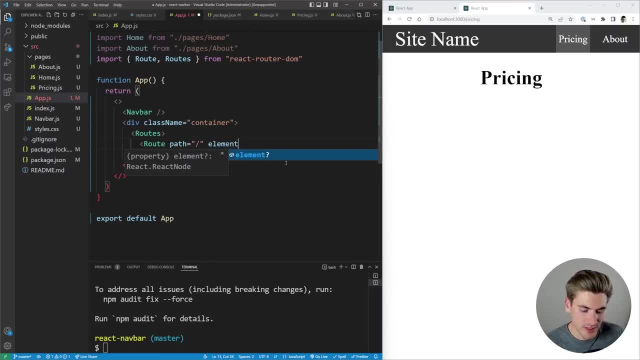 example, is going to be like the index page, and then it's going to have an element, and this is the thing it's going to be rendering out. so in our case, we're rendering out our home component, just like that, and then we can close off that route. so now, this is exactly the same as what? 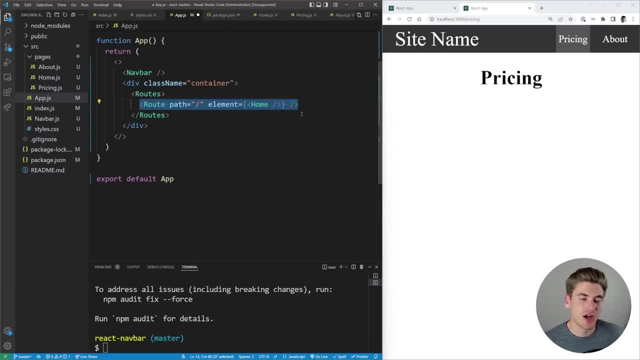 we had in our switch statement, but it's just handled by react router and they have a bunch of other things that they're going to do along with this. so let's just paste this down a couple times. so we have our pricing page and we also have our route component and we're going to 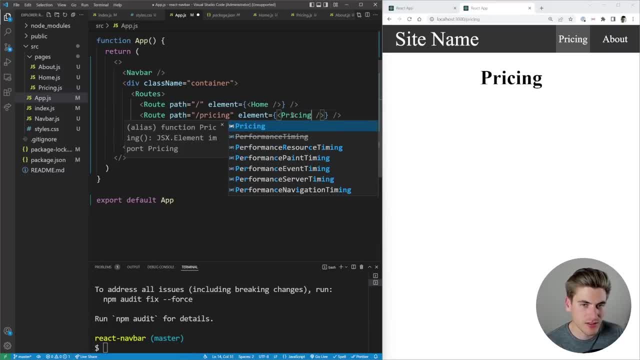 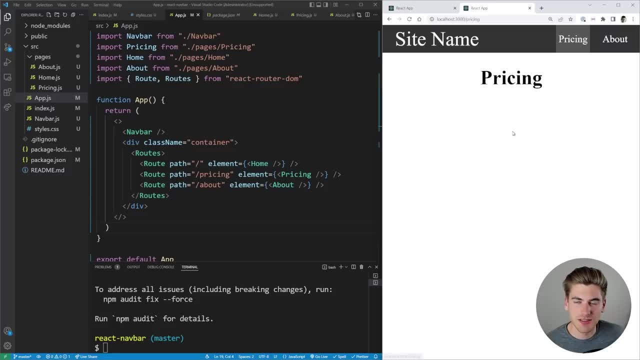 have our about page and our pricing is going to render out pricing and our about is going to be rendering out the about page. so now, if i save and start navigating around, you're going to notice it actually doesn't change anything. it still re-renders the entire page, and that's because 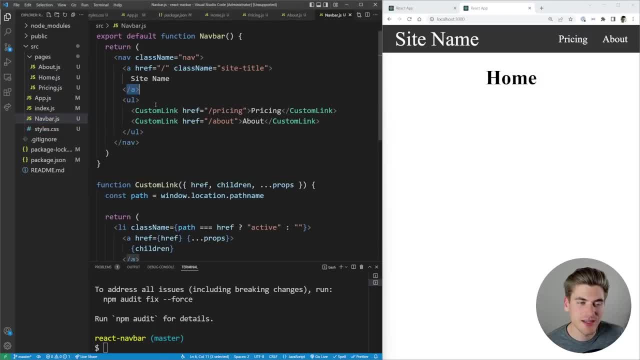 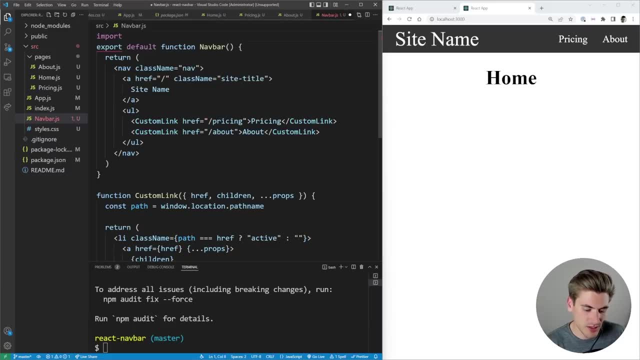 inside of our navbar if we just go to that component. we're using normal a tags. we need to replace this normal a tag with a link component that is from react router at the top. here we're going to be importing the link component from react router dom and this link component. essentially we're 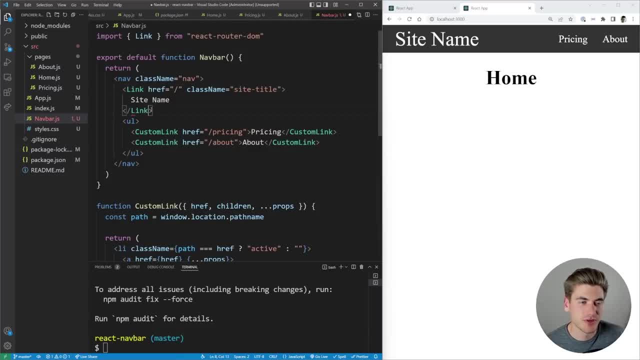 going to be using the link component from react router at the top and we're going to replace it with a link component, and this link component replaces our anchor tag. so anywhere that you see an anchor tag, we want to replace this with a link. same thing down here we're going to replace. 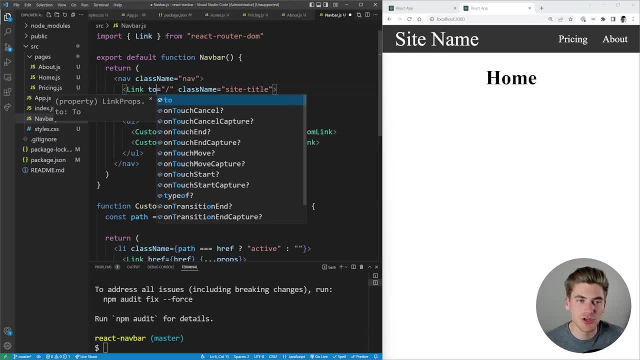 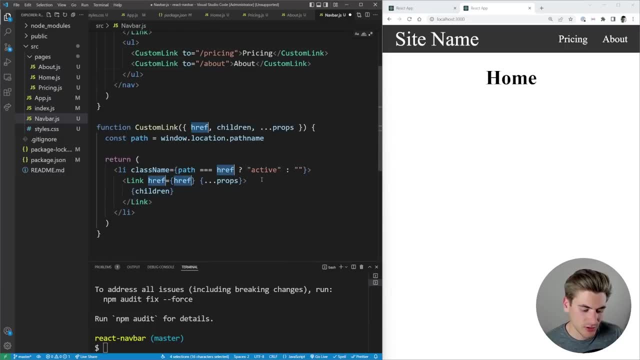 this with a link. but what's really important is that, instead of using href, we're using the word 2.. essentially, wherever you have an href inside of this, you're going to replace it with 2 and it's going to work exactly the same. so in our custom links, we're also going to replace these with 2. 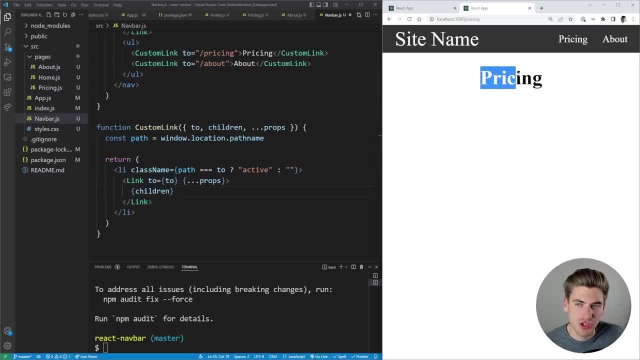 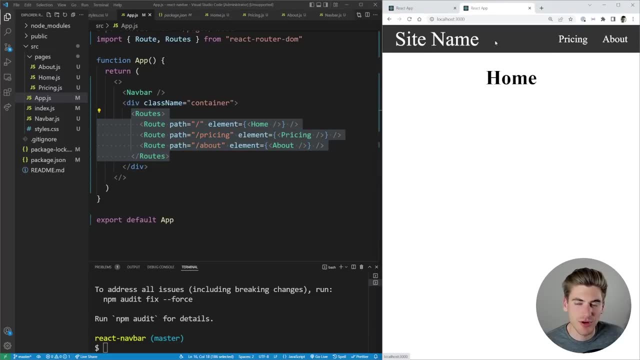 and inside of here we're going to replace all instances of href with 2.. so now, if i save this changing, so if we go back to our app, only the section inside this, routes, is changing and everything else stays the same. so our nav bar stays exactly the same, our container here stays. 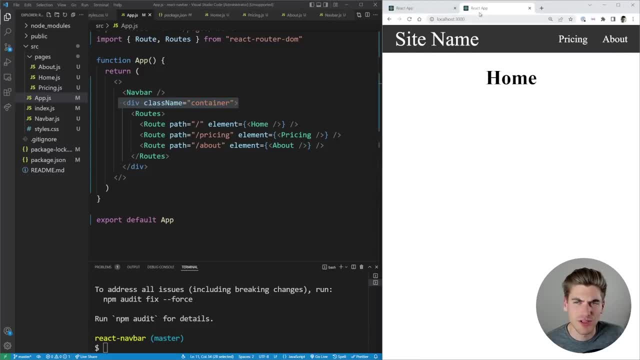 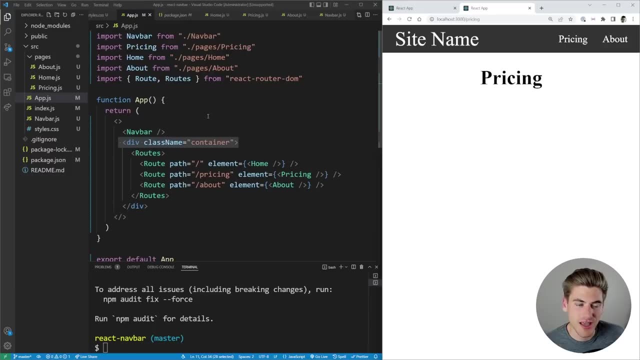 exactly the same and again only this one section changes and our navigation bar up here at the top changes. but you'll notice that our actual active classes don't work and that's because our page never refreshes at all, so our window dot location isn't really changing. so if we go to our nav bar, 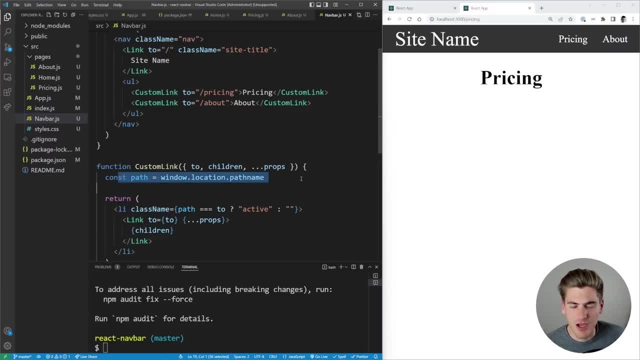 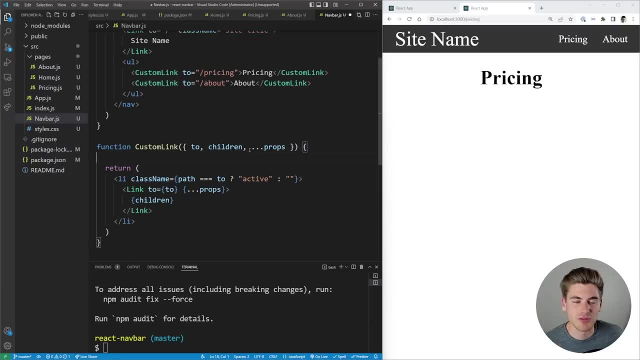 here. this path right here is not actually 100 correct and we can't really rely on this for this. so instead you need to use react router's way of handling this, and they have their own custom hooks you can use to make this work really well. the main hook that you want to care about is the use match. 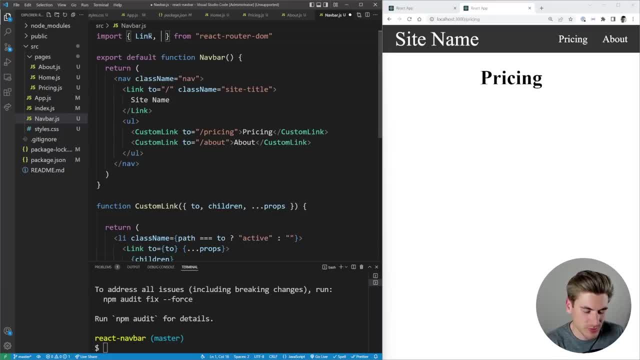 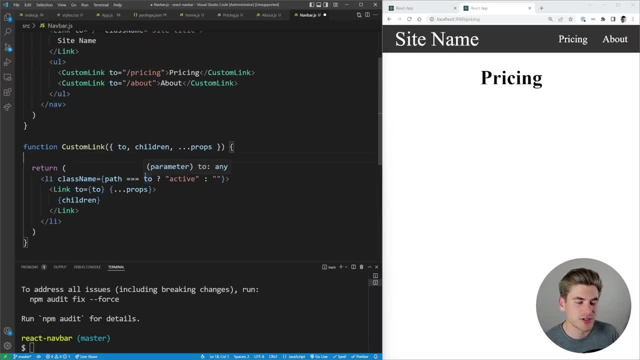 hook, but we're also going to be using a hook called use resolved path. so let's make sure we get that use match hook and use resolved path, and i'll tell you exactly why you need both of these in just a second. so use match allows us to compare essentially the current path that we are on to. 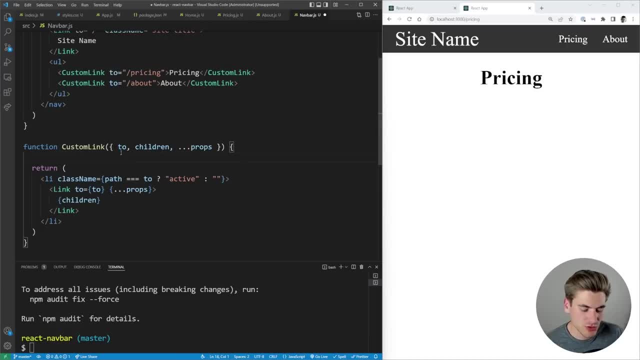 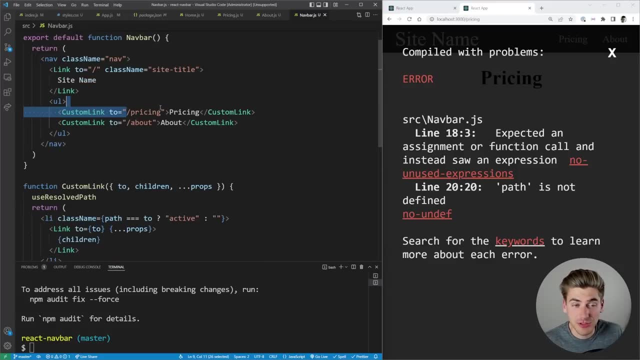 whatever path we want so we can compare it to this to property and used resolved path. this is really important because the way the router actually works with react router and with normal link tags is you can have absolute paths like this which are like absolute. you start with this forward slash and you go to the pricing page, or you could have relative links that say you: 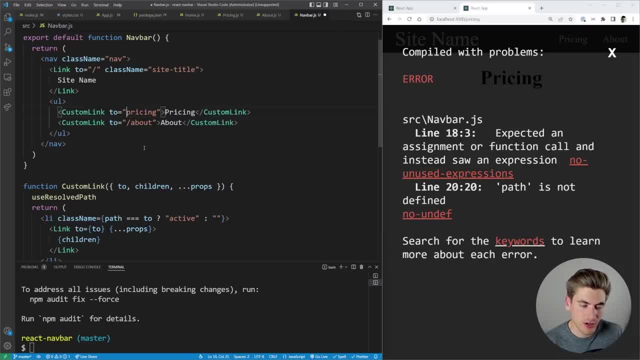 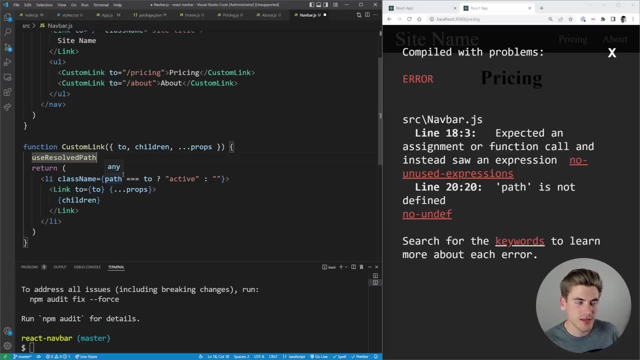 know what, go to the pricing page, relative to whatever page you're currently on. so this use resolve path essentially allows you to take a relative or absolute path. it combines it with the current path you're on and gives you the actual full path that you would be accessing. 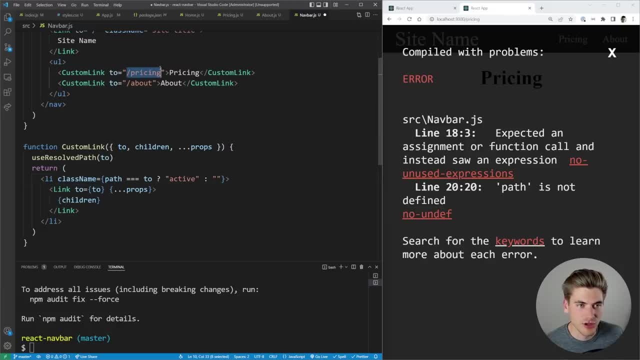 so we're just going to pass in our to property here, which is essentially our url that we're navigating to, and we're going to get that resolved path and essentially, like i said, this converts these relative paths to absolute paths and so on. with absolute paths it's. 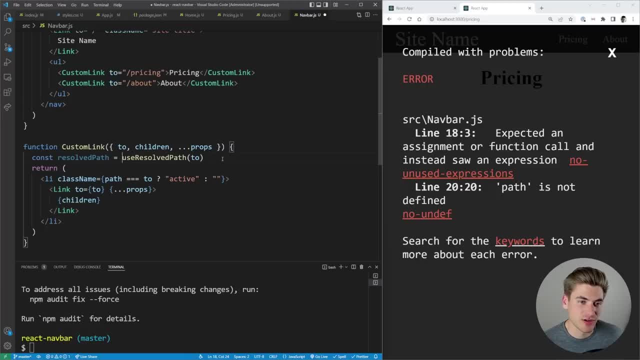 just going to make sure that your path is the full absolute path, even if it starts out relative, and then we can determine if this is active by just saying we want to use that match class. so we could say: use match and this use math. you can pass it a string or you can pass it in. 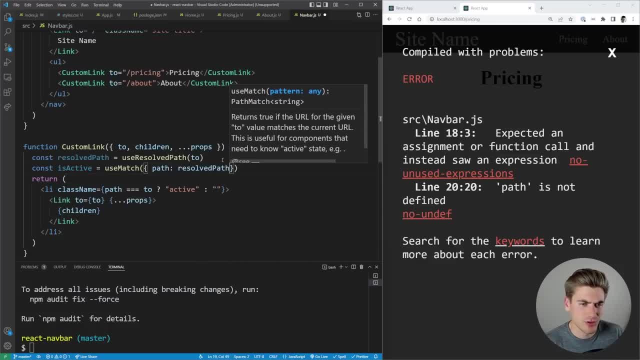 essentially an object and with the object we want to pass a path which is our path name for our resolved path. that's the same thing as, like, windowlocationpathname. and then i want to pass an end of true by saying n true, we just essentially are saying that the entire path, much must match. 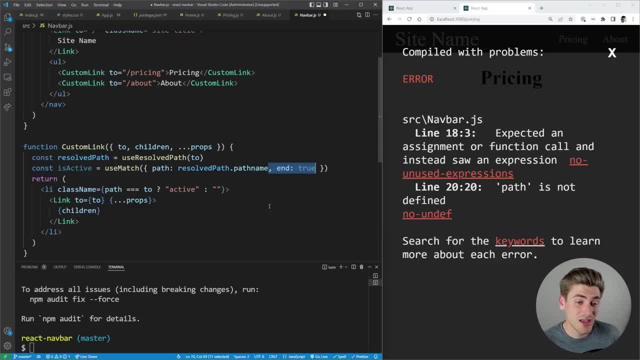 because with react router you can actually do like partial matching and in our case we want to make sure that the entire url is exactly the same. we don't want to worry about partial matching. so this would you know be useful, for example, if you had like slash pricing if our current url is.